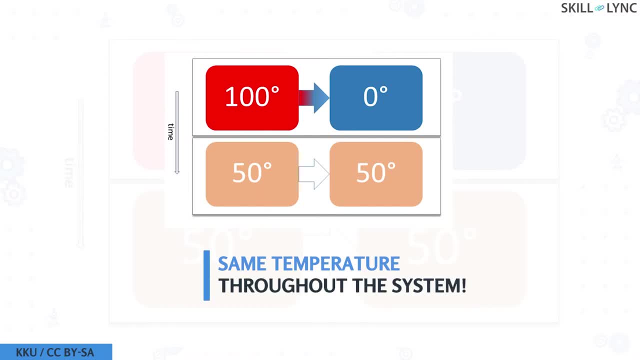 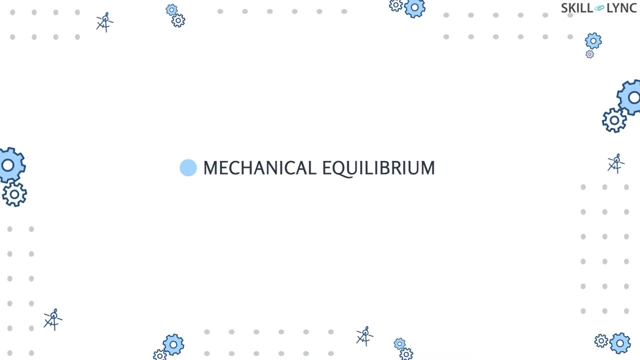 be in thermal equilibrium when the temperature of the system does not change with time and this temperature is the same throughout the entire system. Just like thermal equilibrium, there are mechanical and mechanical temperatures. A system is said to be in mechanical equilibrium when there are no unbalanced forces acting. 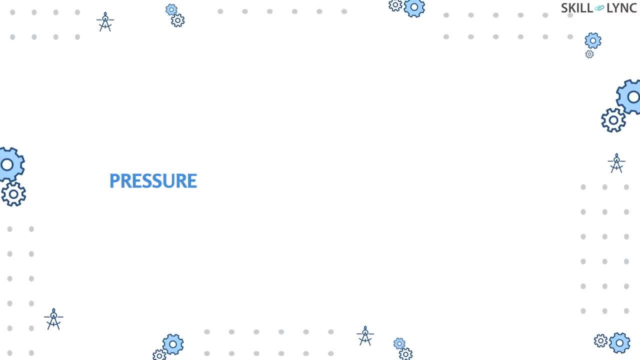 within the system or between the system and the surroundings. In such an equilibrium, the pressure is the same at all points in the system and it does not vary with respect to time. On the other hand, a system is said to be in chemical equilibrium when there is 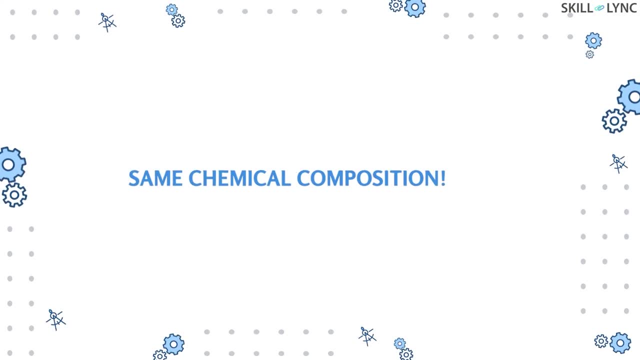 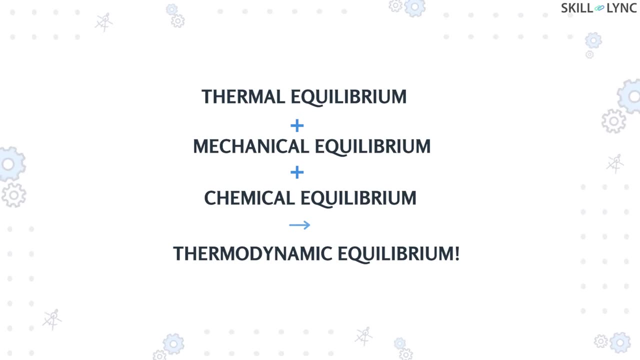 no chemical reaction taking place in the system. The chemical composition is the same throughout the system and does not change with respect to time. A system which has two bodies is called a chemical equilibrium, A system that is set to be in thermodynamic equilibrium when the temperature and pressure is the same at all. 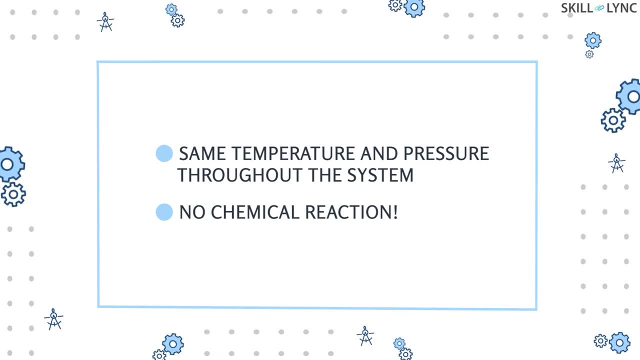 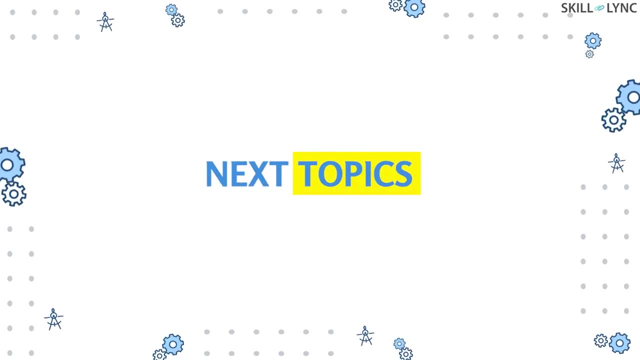 points in the system and there is no chemical reaction taking place within the system or between the system and the surroundings. That's all for thermodynamic equilibrium. Now let's move on to our next topics, which are state path and process. We know that the condition of a system varies from time to time, The more the system is. 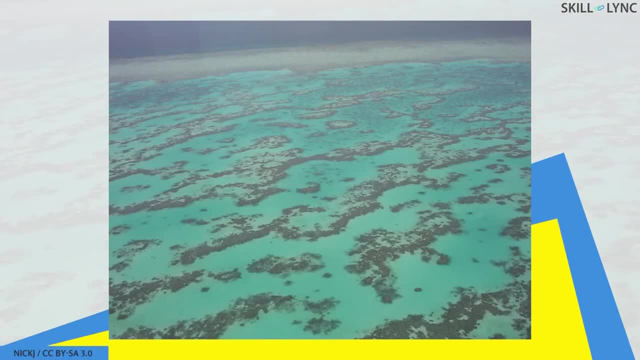 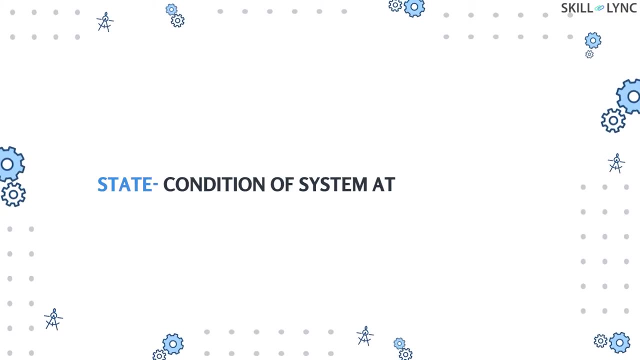 set to be in thermodynamic equilibrium, the more it will change. The most common example is the environment. Considering the environment as a system, the environmental conditions never stay the same. In thermodynamics, the condition of a system at a given point of 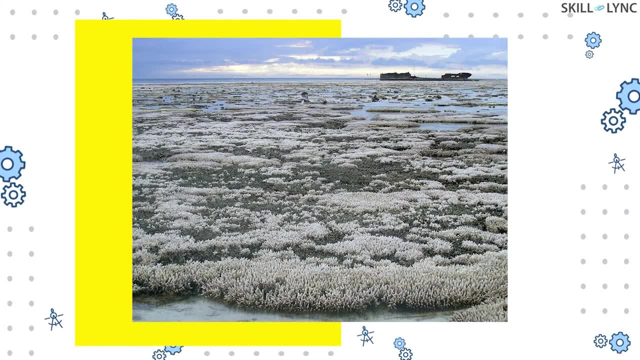 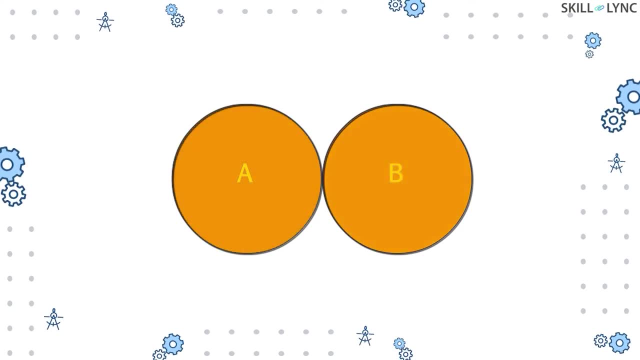 time is termed as a state. In simpler terms, each unique condition of a system is called a state. We know that a system passes through several states to reach an equilibrium. Moreover, a system passes through several more states in order to move from one equilibrium to another. 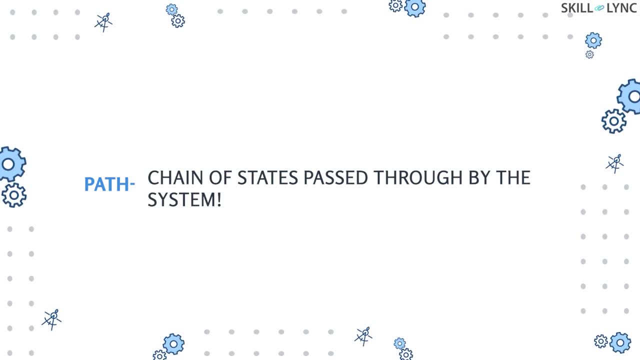 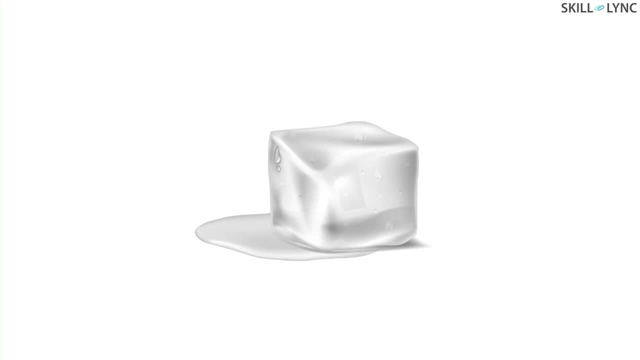 The chain of states passed through by a system as it moves from one equilibrium state to another is called the path covered by the system, And when a system goes through changes from one thermodynamic state to another, due to changes in properties like pressure and temperature, then the system is said to have undergone a thermodynamic process. 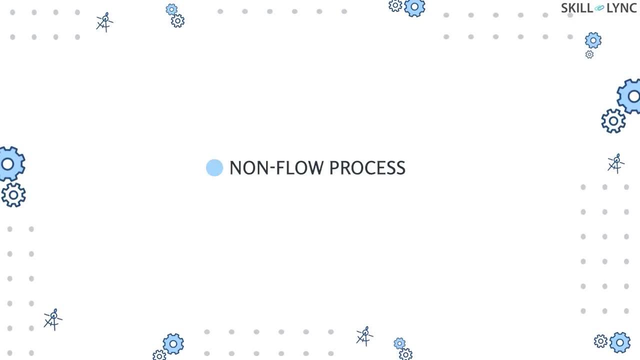 There are two types of thermodynamic processes, namely non-flow process and flow process. In a non-flow process, only energy enters and leaves through the boundaries of the system. On the other hand, in the flow process, both mass and energy enter and leave through the boundaries.